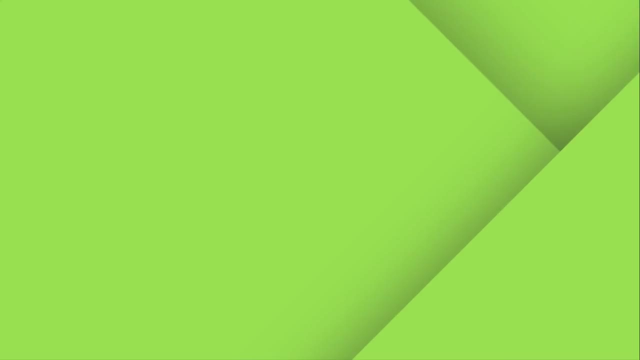 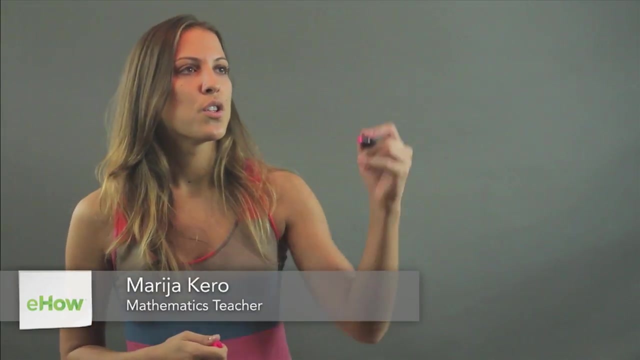 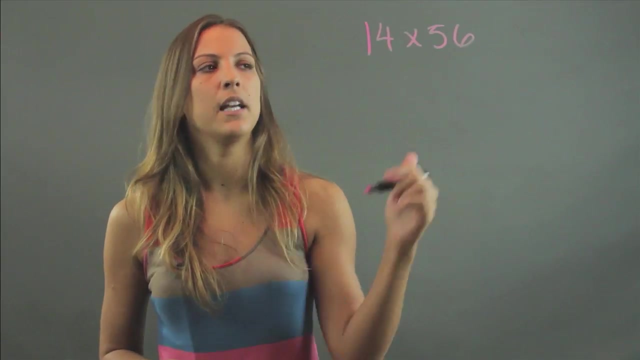 Hi, my name is Maria, I'm a mathematician and today I'm going to show you the lattice method of multiplication. So we're going to take a multiplication problem like 14 times 56, and instead of setting it up the traditional way- the 56 under the 14,- we're going to set 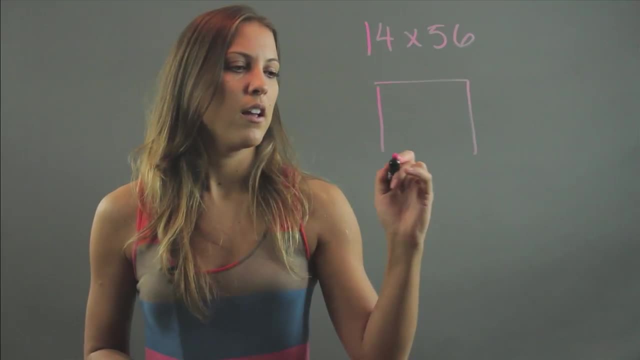 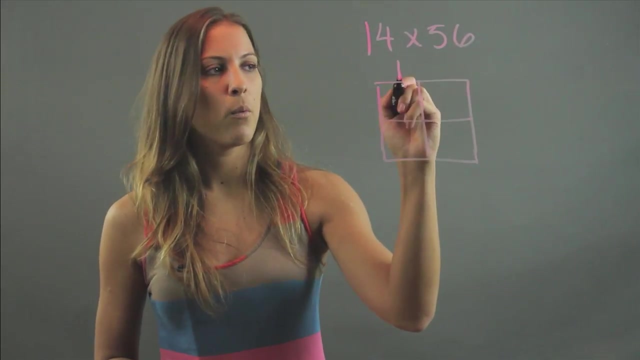 up lattice. So for lattice, we're going to have to draw a square and we're going to go ahead and split that square into four equal parts and I'm going to write the first digit up top 14.. I'm going to split it up into its 10th digit and its 1th digit. so it's. 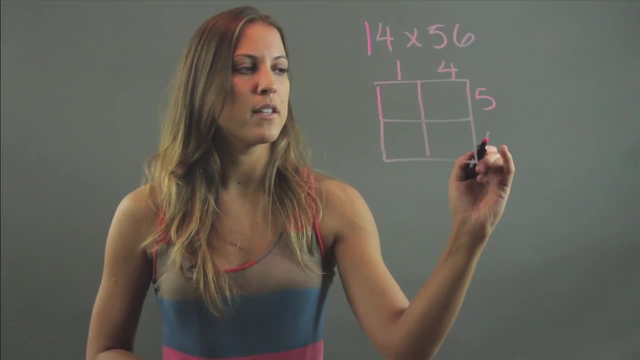 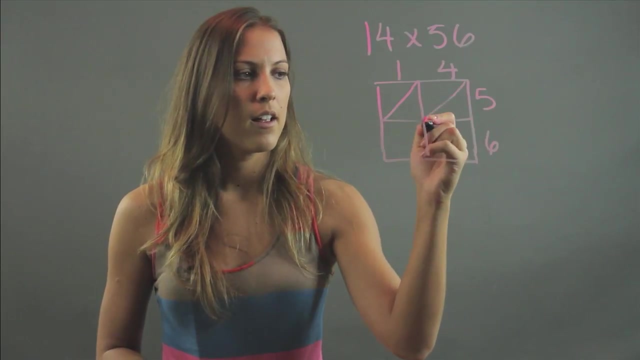 1,, 4, and 56 is going to go ahead and go vertically this way: 56.. Now you're going to have to draw a diagonal within each of the squares in your small squares. So I'm going to go like that, like that, like this and like this. Okay, so I split each of my four smaller 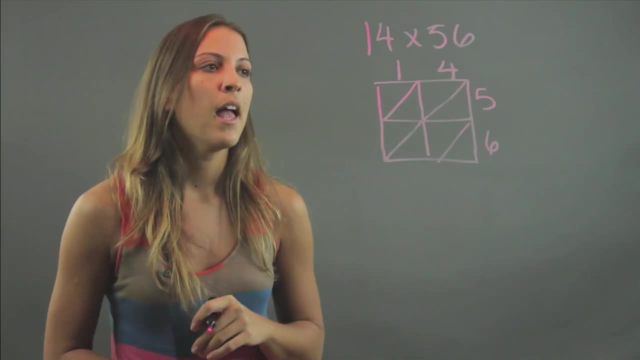 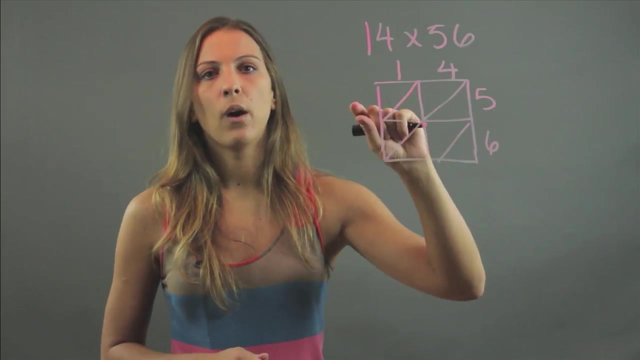 squares into half by splitting diagonals. Now I'm going to go ahead and multiply 1 times 5, and that product is going to go in this cube. Now, what you do is 1 times 5 is 5, right, So it's going to go 0, 5.. So you put the 10th. 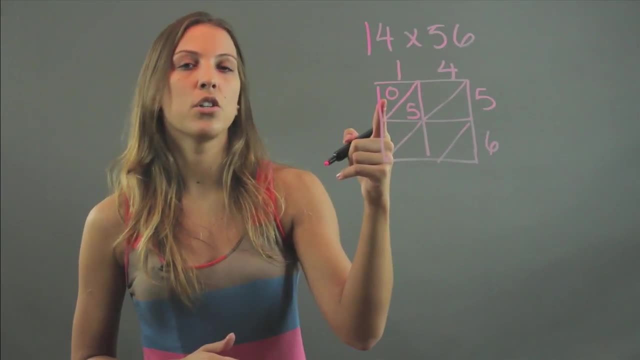 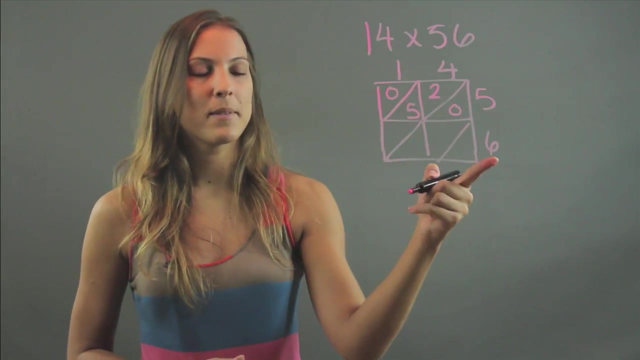 digit and then the 1st digit. but because there is no 10th digit here, you just put a 0. 4 times 5 is 20, so I'm going to put the 10th digit and the 1st digit 1 times. 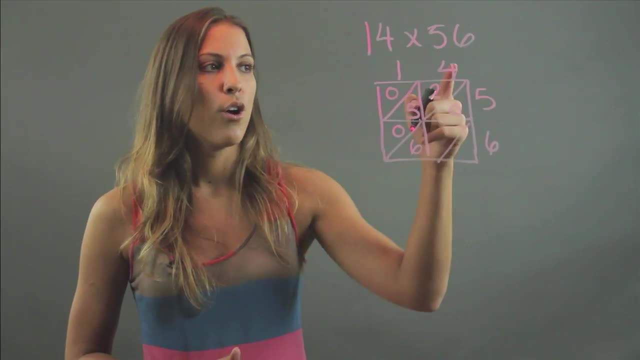 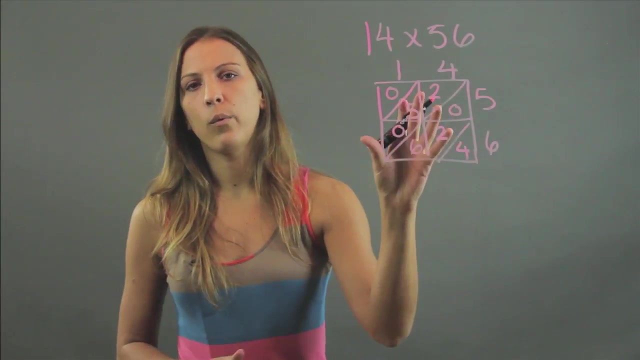 6 is 6, so it's just 0, 6.. 4 times 6 is 24, so 24.. 10th digit, 1st digit. Okay, now, when all of your multiplying within the square is done, what we're going to do is some addition. 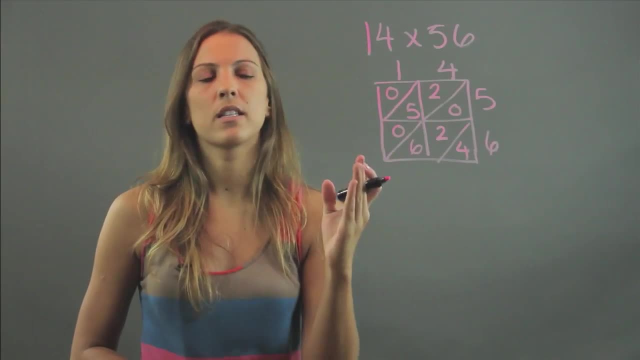 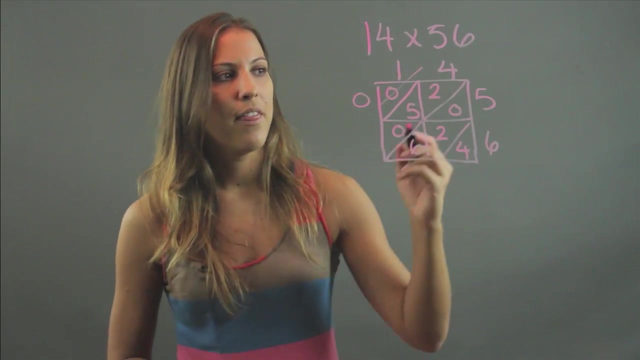 You're going to add along the diagonals. So the diagonals come this way right. So I'm going to add all the numbers going this way, which is just the number 0, so obviously that's just going to be 0. Then I'm going to add 2,, 5, and 0. I'm adding all the numbers along. 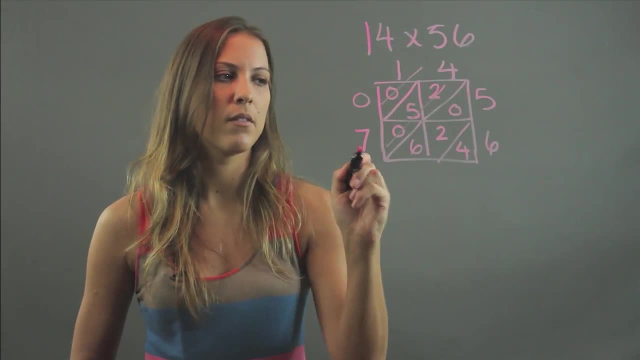 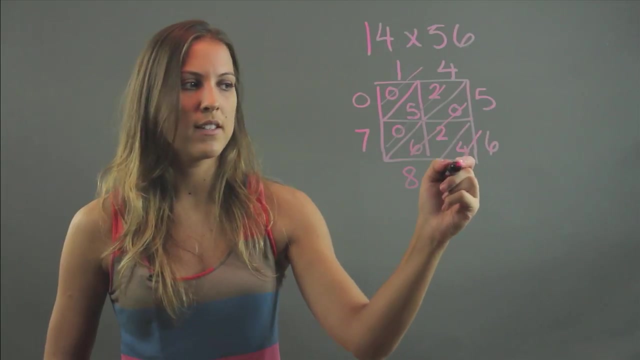 that diagonal 2 plus 5 is 7, plus 0 is still 7.. Now I'm going to add along this diagonal: 0 plus 2 plus 6 gives me 8.. Along this diagonal is only this number, so it's just 4.. Now when 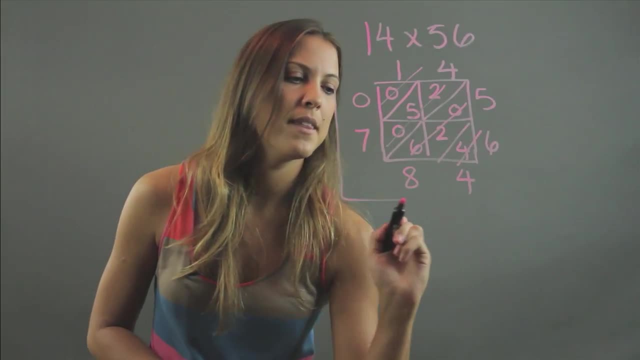 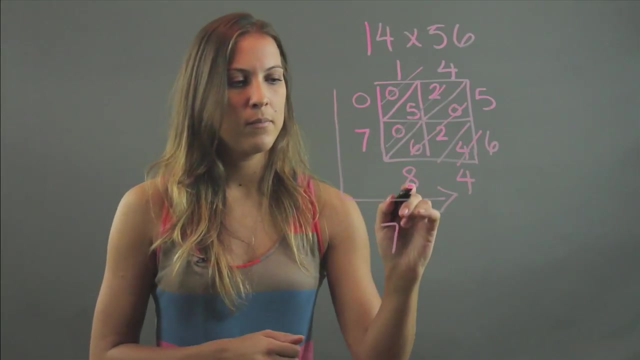 you're done. adding your solution is going to be 1 times 4 times 4 times 5.. So you're read this way as an L. So we're going to start with a zero, which I don't need, because as a leading number I don't need a zero. So I'm going to write 7,, 8,, 4.. The 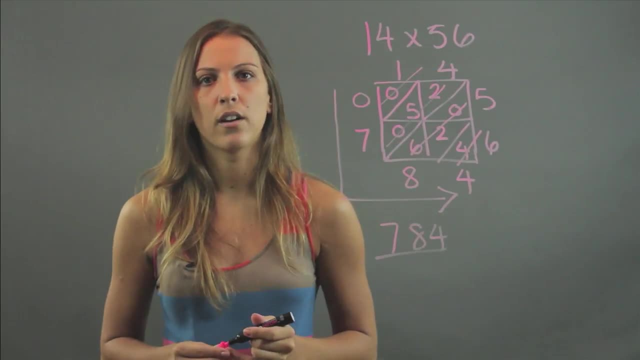 product of 14 and 56 is 784.. My name is Maria and I just showed you how to do the lattice method of multiplication. 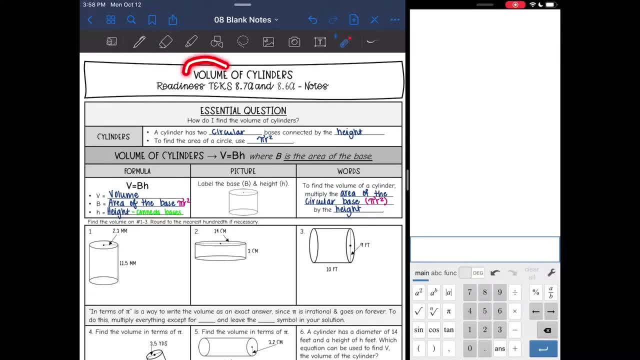 Hey everyone, we are starting to look at volume today. Remember, volume is how much space a figure holds, how much space a 3D figure takes up. So we're going to look at the volume of cylinders and we are going to be finding how much space is inside the cylinder. So, reminder of cylinders. 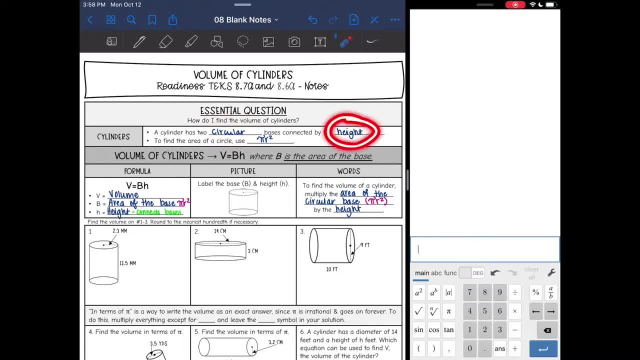 they have two circular bases that are connected by the height, and their circular bases we're going to have to find the area of them. So, reminder: to find the area of a circle you use pi or squared. So here is the volume of a cylinder formula. It is: V equals capital B times H, where capital B 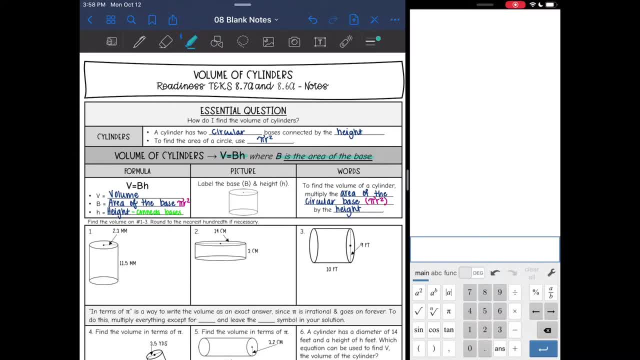 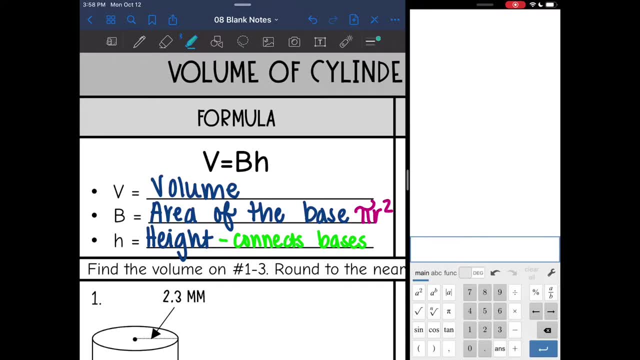 is the area of the base. So let's break that down a little further here. Here's our formula: V equals BH, V is the volume capital, B is the area of the base. So we're going to have to find the area of the circular base by using pi R squared. So that means I will replace the B. 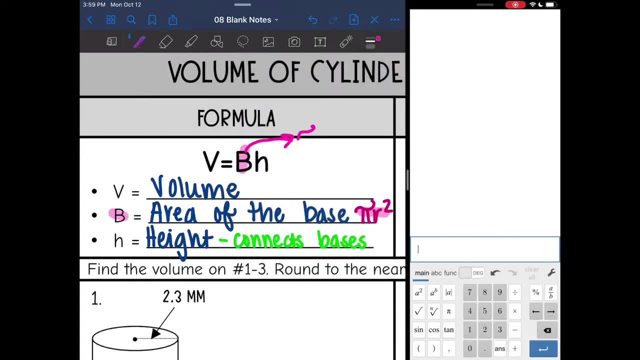 with the area of the base. So that means I will replace the B with the area of the base. So that means I will replace the B with whatever pi R squared is, And then I will multiply it by the height of the cylinder, which, remember, is the distance that connects the bases. 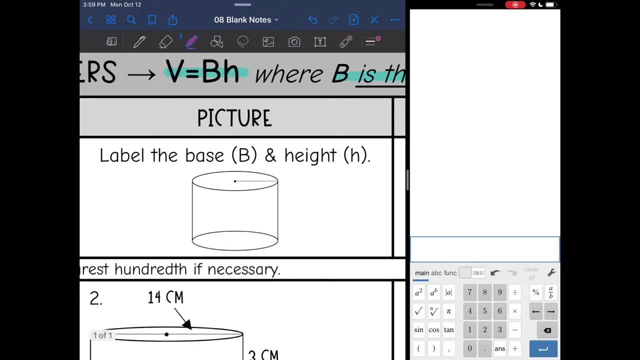 So let's look at those a little bit closer. here. Capital B is our area of the base, So I'm going to find the area of those circles And then my height is the distance that connects those. So this distance right here, those are the two things that we're going to need.